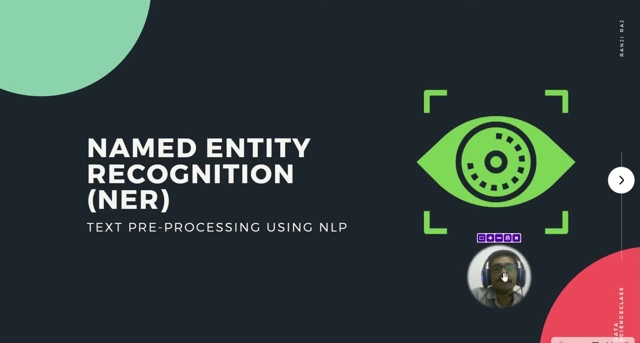 Hello people, welcome back to my channel. So in today's video we'll be seeing about what is named entity recognition, that is, NER in NLP. So so far we have discussed about what is POS, tags, chunks and different things. So NER is one of the last component in NLP. Thereafter we'll be doing different applications and other techniques we'll be discussing. 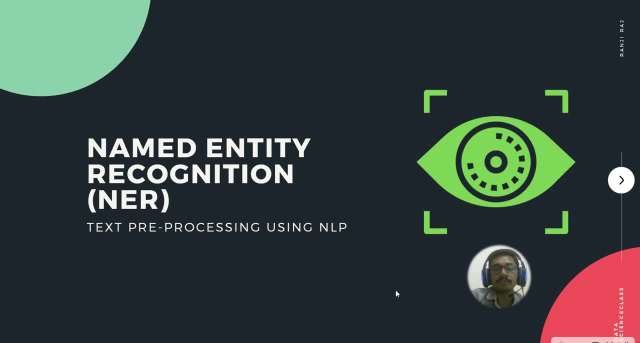 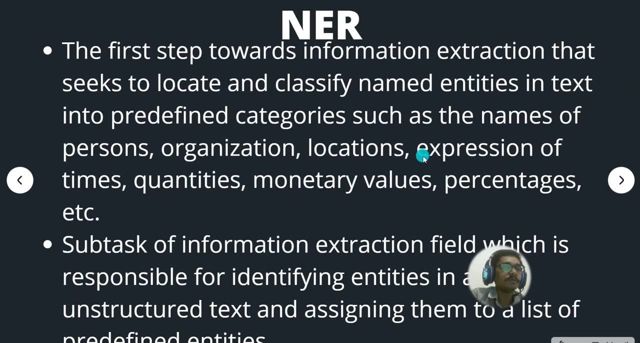 So NER is one important thing that you have to keep in mind when you deal with NLP. So let's get started. So what is this NER? So the first step towards information extraction is that to seek and locate and classify the named entities in the context into predefined categories, such as the names of persons, organizations. 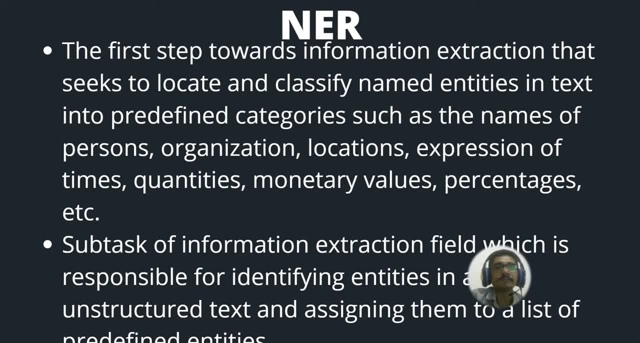 communications, expressions of times, quantities, monetary values, percentages, etc. So it's like whenever you read a particular documentation or something online for a specific topic, say, in the recent times, you have this WhatsApp issue that is going on with privacy issues. So most of the people would search for about the history of WhatsApp and its relationship with Facebook, when they bought it, for how many years. So that's what we're going to be discussing, So let's get started. 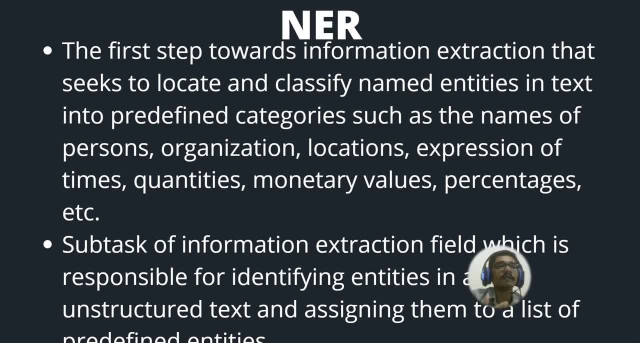 So in that context, you will have different names of different persons that will be coming CEO of Facebook, the quantities, that is, the monetary quantities, and how much US dollars it was bought in which year and how much was the GDP and all those things. So, based upon the different locations, you'll get this many information So you can actually collate these words and you can relate to one particular entity. So that is what we're going to be discussing. 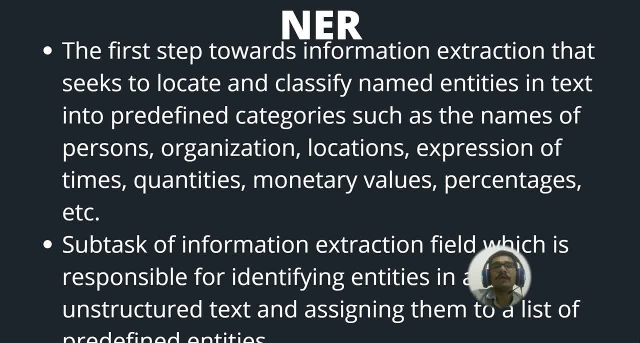 So in that context, you will have different names of different persons that will be coming CEO of Facebook, the quantities, that is, the monetary quantities, and how much US dollars it was bought in which year and how much was the GDP and all those things. So, based upon the different locations, you will get this many information. So let's get started. 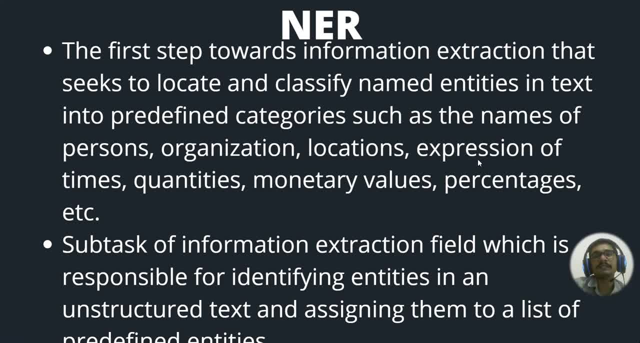 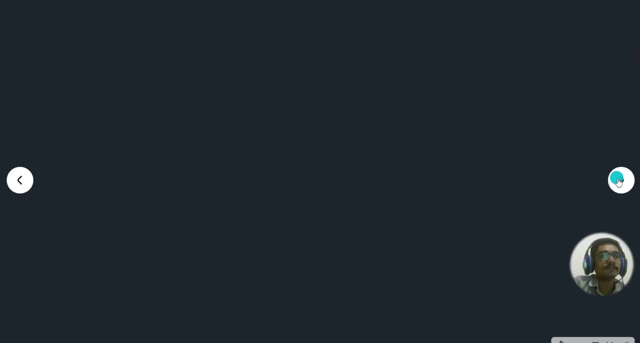 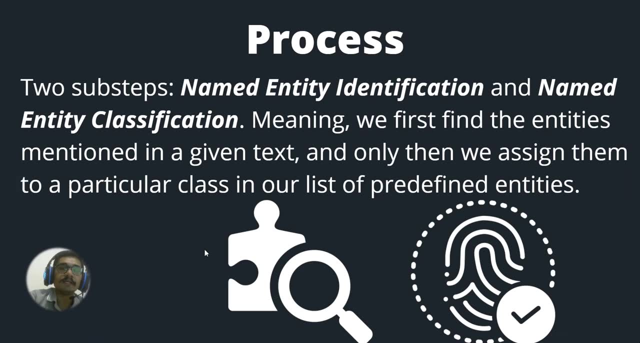 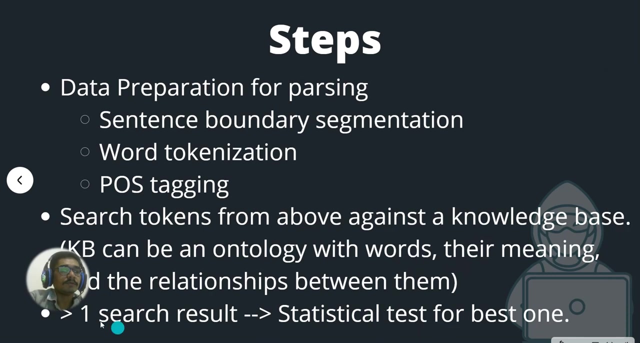 So in that context, you will have different names of different persons that will be coming: CEO of Facebook, the quantities- that is, the monetary quantities, and how much was the GDP, and all those things. So let's get started. So in that context, you will have different names of different persons that will be coming CEO of Facebook, the quantities- that is, the monetary quantities, and how much was the GDP, and all those things. So let's get started. 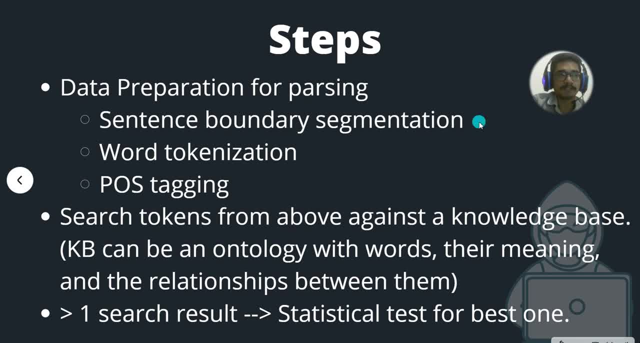 So in that context, you will have different names of different persons that will be coming: CEO of Facebook, the quantities- that is, the monetary quantities, and how much was the GDP, and all those things. So let's get started. So in that context, you will have different names of different persons that will be coming CEO of Facebook, the quantities- that is, the monetary quantities, and how much was the GDP, and all those things. So let's get started. 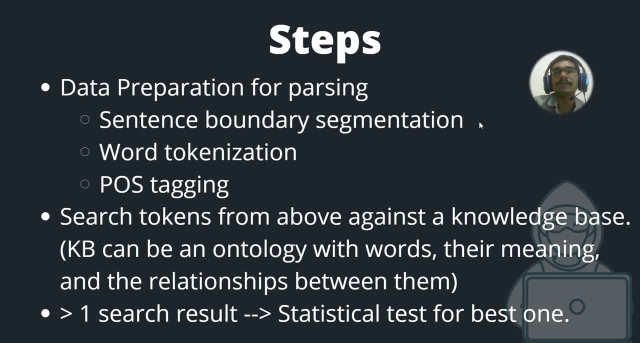 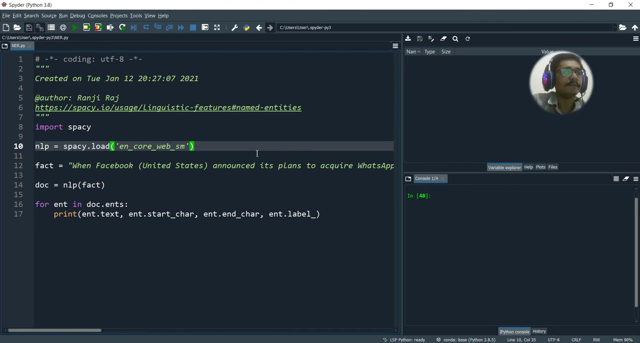 So in that context, you will have different names of different persons that will be coming: CEO of Facebook, the quantities- that is, the monetary quantities, and how much was the GDP, and all those things. So let's get started. So in that context, you will have different names of different persons that will be coming CEO of Facebook, the quantities- that is, the monetary quantities, and how much was the GDP, and all those things. So let's get started. 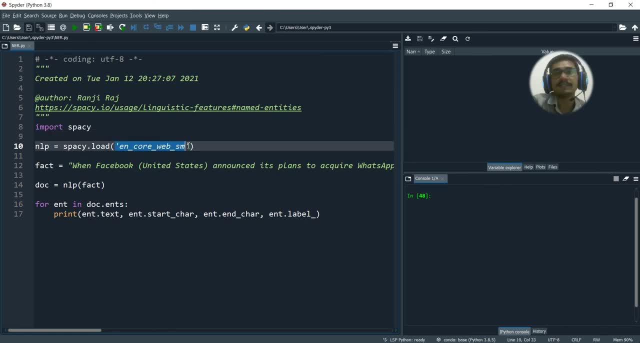 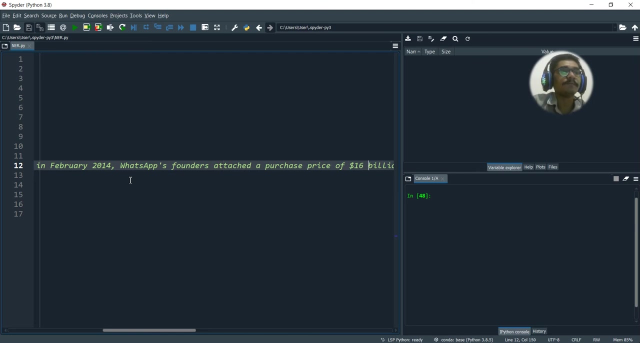 So in that context, you will have different names of different persons that will be coming: CEO of Facebook, the quantities- that is, the monetary quantities, and how much was the GDP, and all those things. So let's get started. So in that context, you will have different names of different persons that will be coming CEO of Facebook, the quantities- that is, the monetary quantities, and how much was the GDP, and all those things. So let's get started. 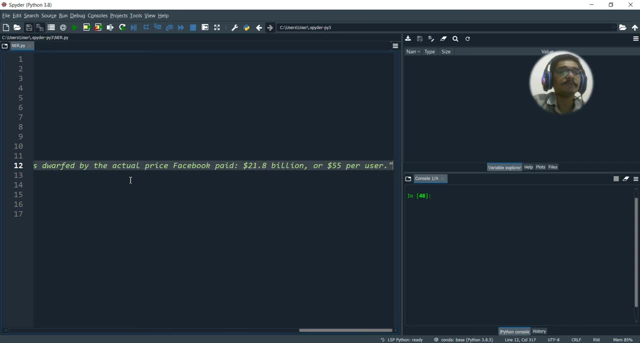 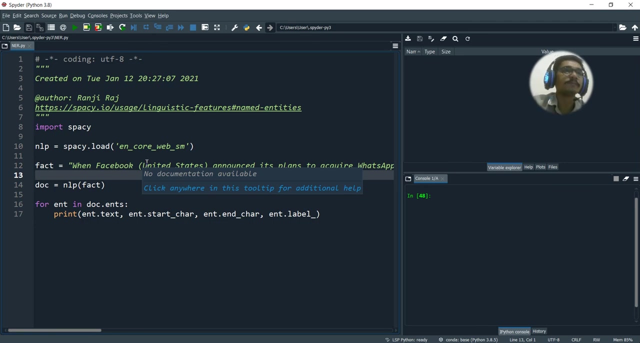 So in that context, you will have different names of different persons that will be coming: CEO of Facebook, the quantities- that is, the monetary quantities, and how much was the GDP, and all those things. So let's get started. So in that context, you will have different names of different persons that will be coming CEO of Facebook, the quantities- that is, the monetary quantities, and how much was the GDP, and all those things. So let's get started. 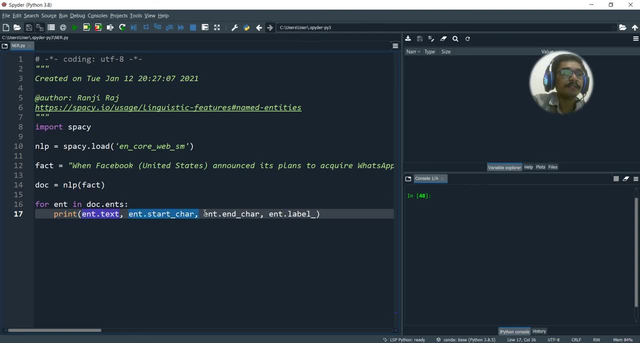 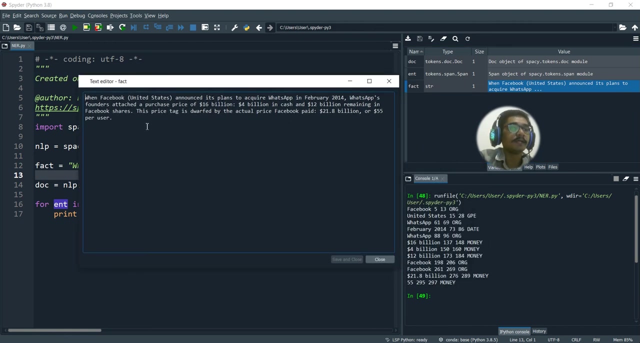 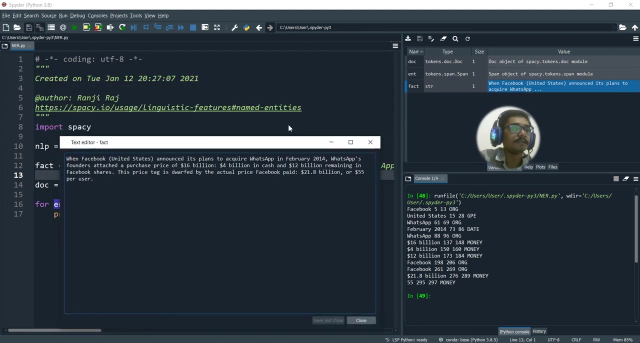 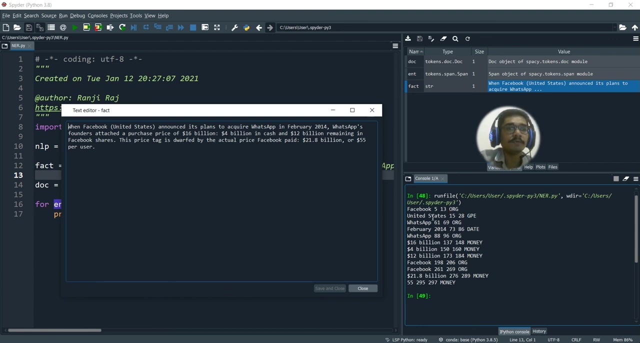 So in that context, you will have different names of different persons that will be coming CEO of Facebook, the quantities- that is, the monetary quantities and all those things. So let's get started. So in that context, you will have different names of different persons that will be coming CEO of Facebook, the quantities- that is, the monetary quantities and all those things. So let's get started.